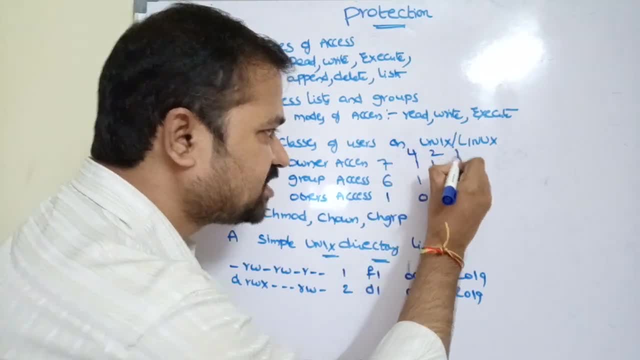 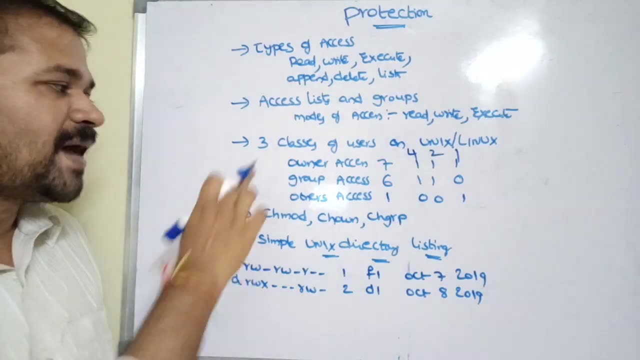 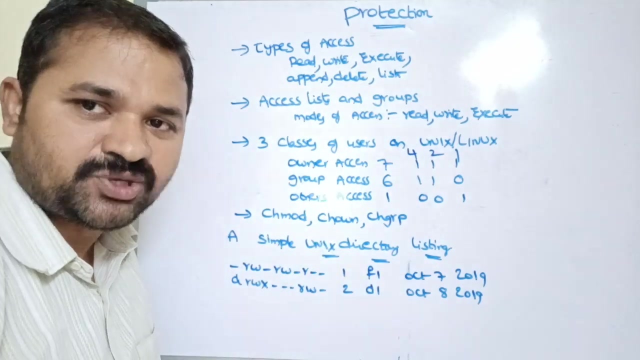 we can have mainly three permissions: read, write and execute permission. so read means four bits, various write means two bits, various execute means one bit. so by default, boner will get all the permissions. why? because boner is nothing but the person who created that file, so he has all the permissions, all. 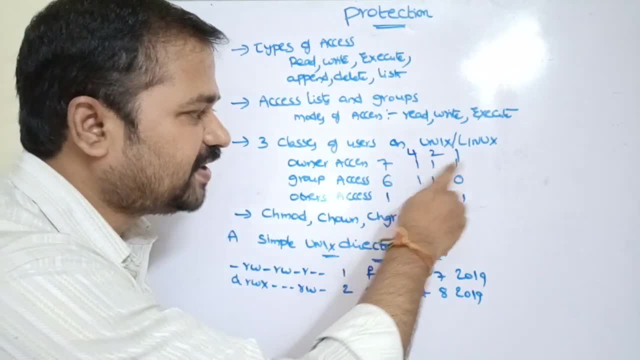 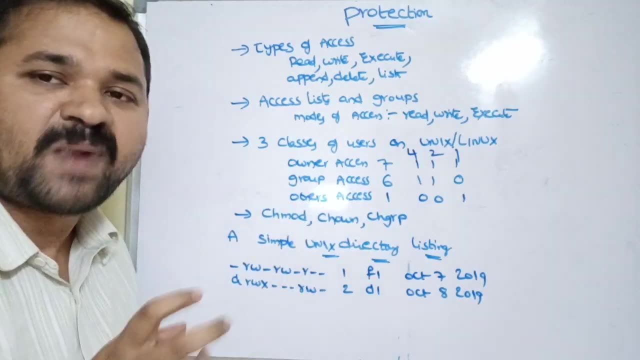 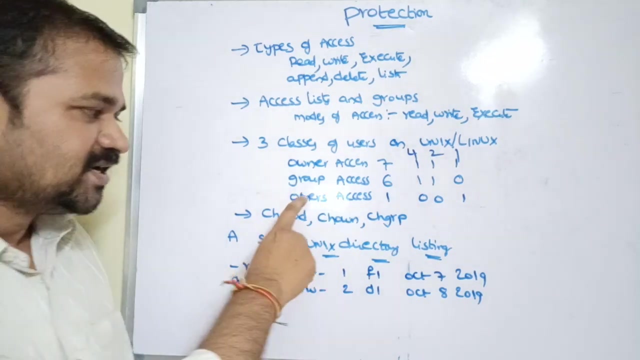 the access permissions on that file. okay, so one, one, one. so four plus two plus one means seven. so boner has seven permissions. next one is group. so by default a group has read permission as well as write permission. so four plus two means six, six bits others by default. others has only execute permission. but 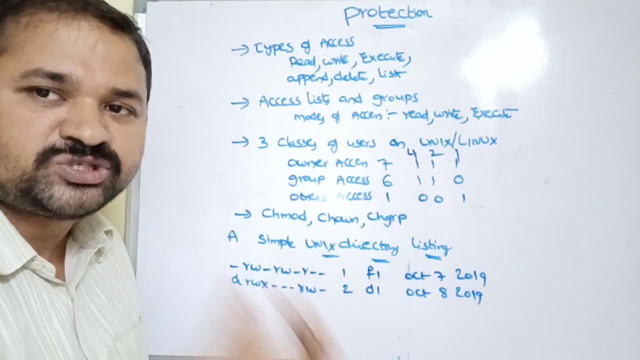 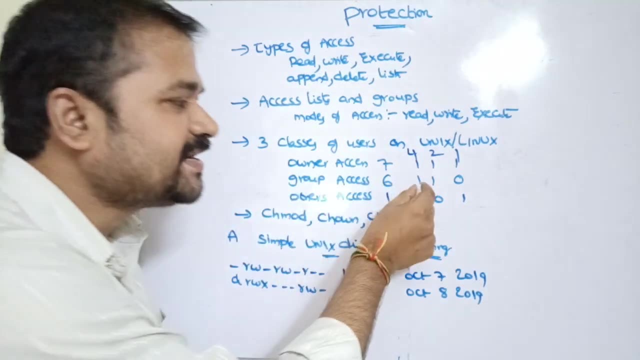 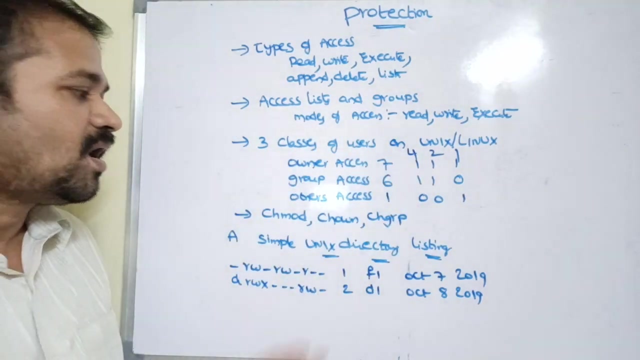 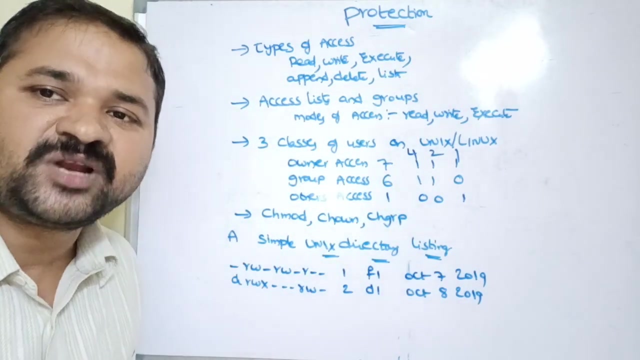 here boner has the ability to change the permissions for the group as well as to change the permissions for the others. so that means boner can release these permissions and boner can give only execute permission for the group, or boner can give read permission and write permissions for the others. so it is the responsibility of 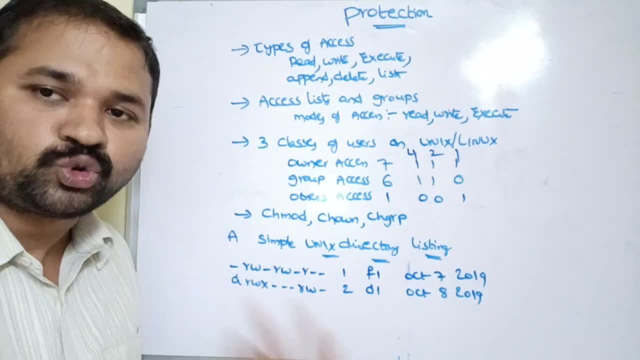 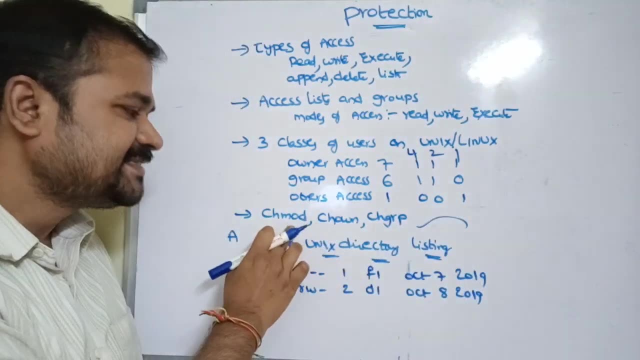 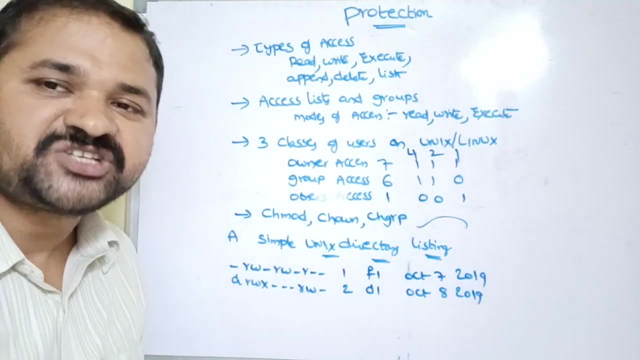 the boner to provide and to release, to remove the permissions for the groups as well as others, that here we have different types of commands. are there ch mode, ch phone, ch group, like that. so ch mode stands for changing mode. so we can change uh mode of your file we can change. 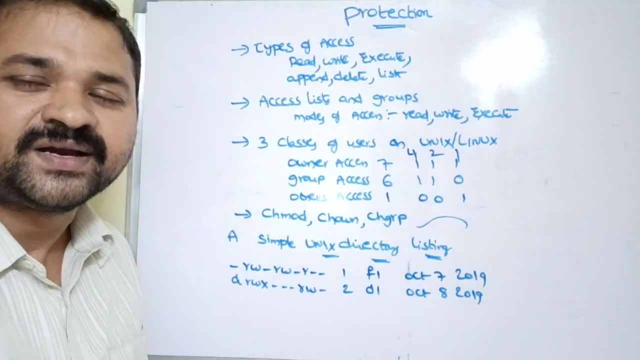 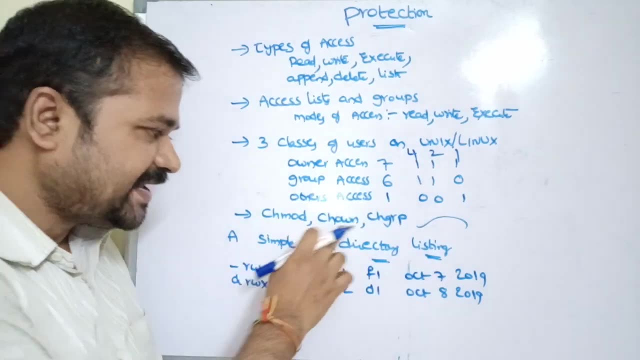 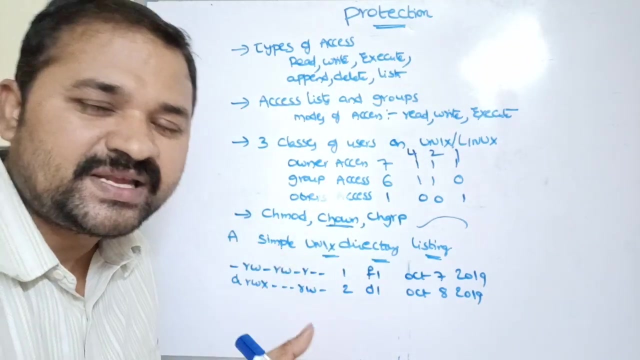 permissions of your file with the help of the ch mode command. generally this command is executed by the boner. why? because boner changes the permissions here. next one is ch one. by using ch one command we can change ownership of a file, so a owner can give that ownership to. 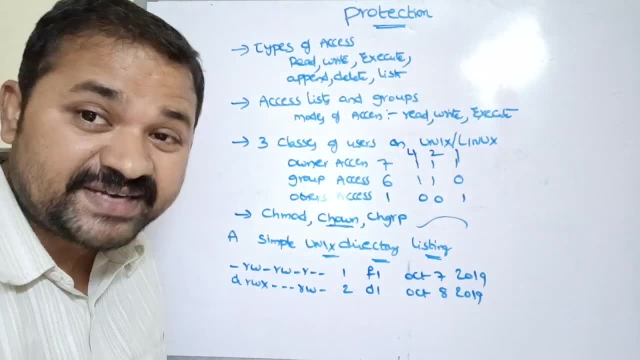 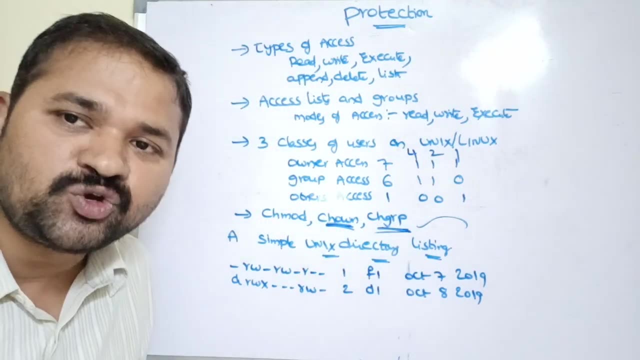 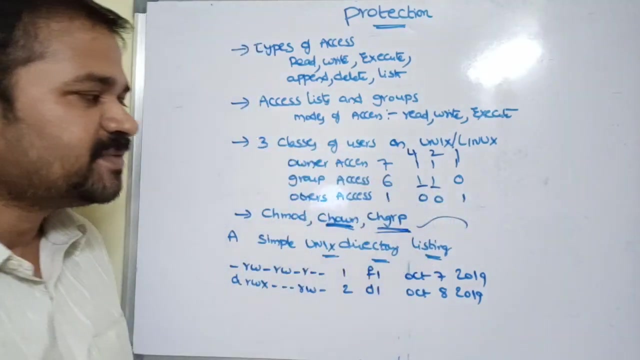 some other person in the group. so in order to change ownership of the file, we can use this ch one. our next one is we have ch group. so by using ch group we can change group permissions of the file. so let us assume that here, initially, only group has read and write permission. 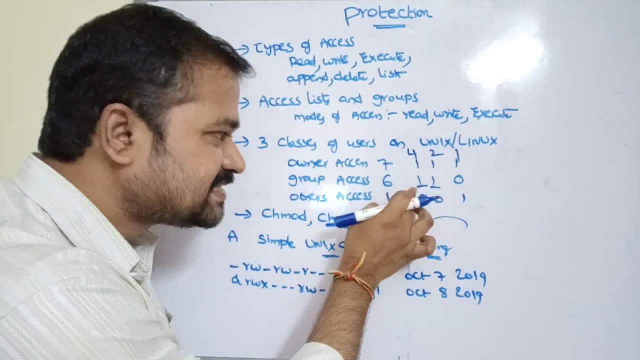 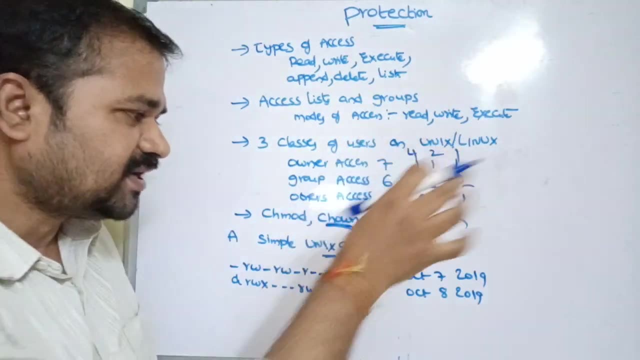 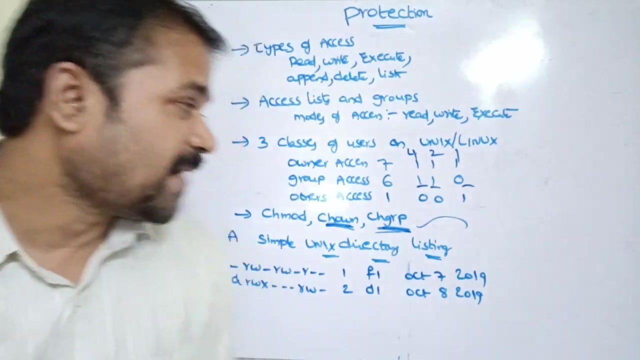 so boner has the permission to change this, read permission, write permission, or boner can give execute permission for a group also, okay, so all that can be happen with the help of ch group and we have umos, so with the help of umos here. by default, boner permissions are seven. 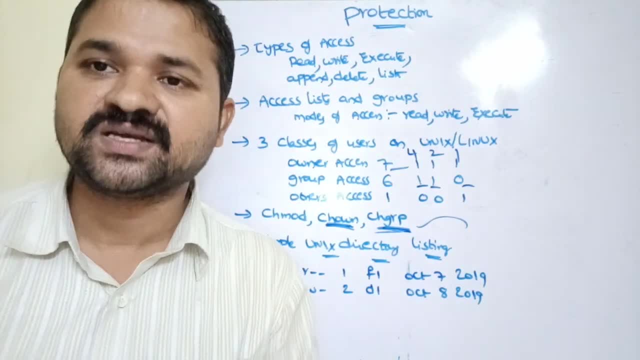 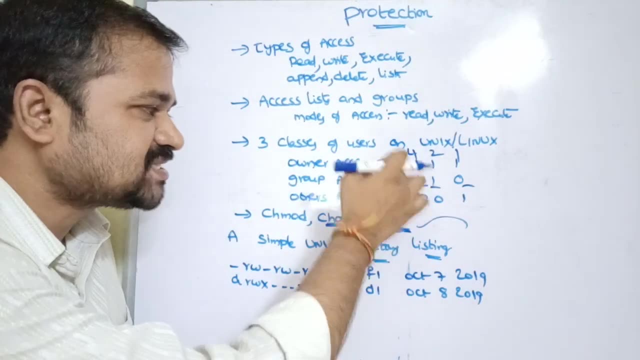 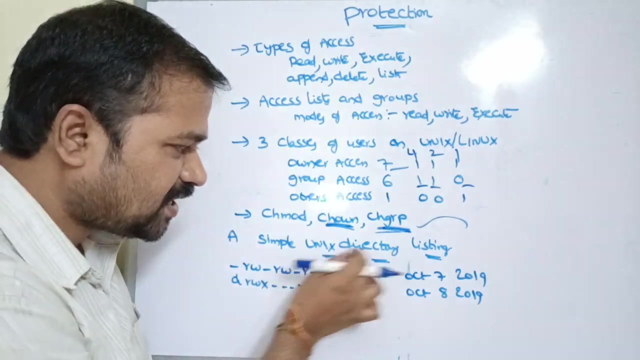 we can change those permissions with the help of umox. so umos is mainly useful in order to change default permissions. okay, so by default the permissions are seven, six one. with the help of umos, we can change those permissions also. uh, next let's see about a simple unix directory listing: uh here. this is nothing but a file where 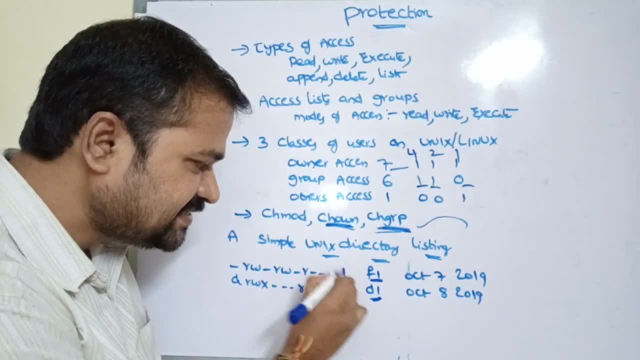 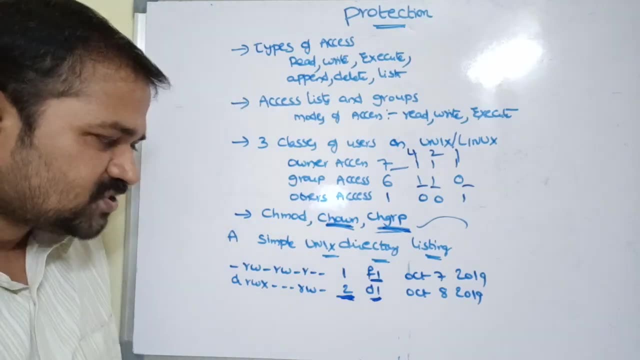 he has. the second one is nothing but a directory. so this one specifies that there is no link here where he has these two. specifies that there is a link here for this directory so that if you perform any modifications on d1, then that modifications will be reflected on. 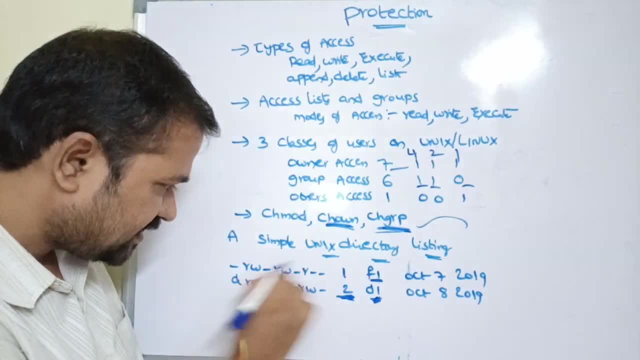 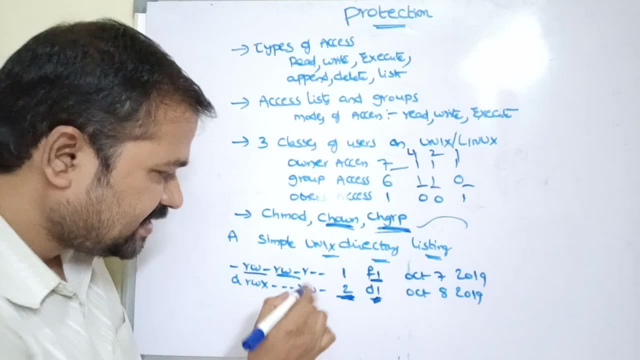 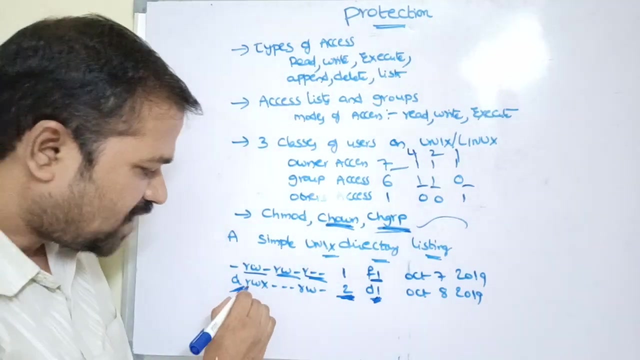 other directory also. okay, uh, it specifies that uh, for f1, boner has only read write permission. where he has group has read write permission. others has only read permission. a directory can be listed with d, so d stands for it is a directory a boner has read permission, write permission. 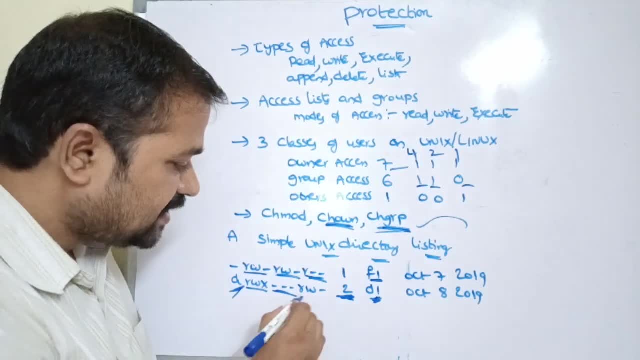 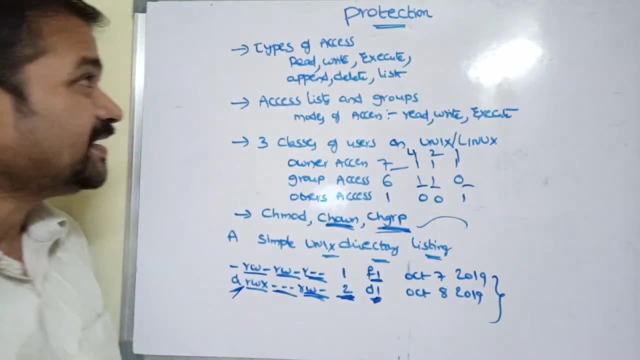 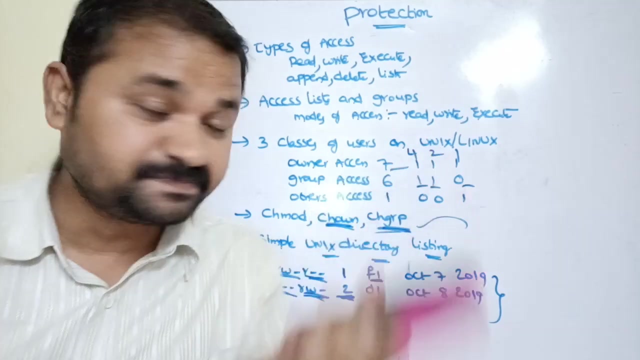 execute permission. a group doesn't have any permission and next others has read and write permission. okay, so it specifies the time and date at which the file is created. okay, so with these mechanisms we can provide protections to files on unix or linux operating system. so if you don't provide a protection mechanism, then there is a possibility that 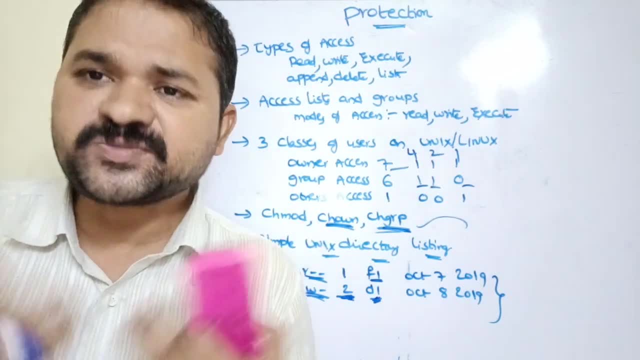 other persons may access our data, so we must provide protection mechanism so that other persons cannot access our data. so this is about file protection.